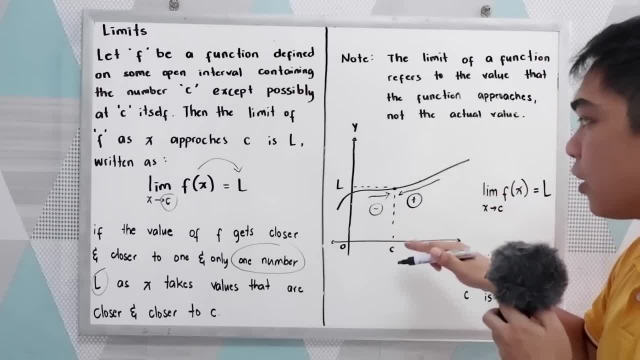 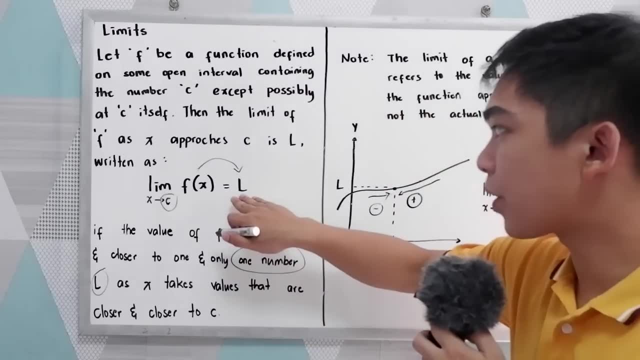 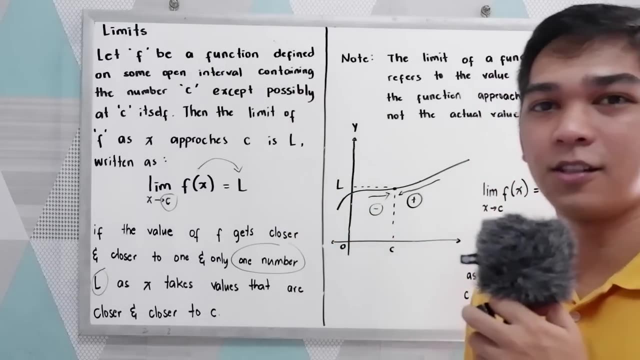 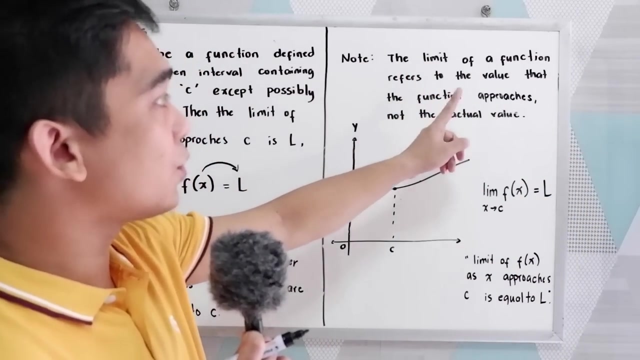 the positive numbers will be our second area. Those are the things that we need to consider, Because if our l is different, that will give us that the limit does not exist. To understand this, let's have our node here. The limit of the function refers to the value. 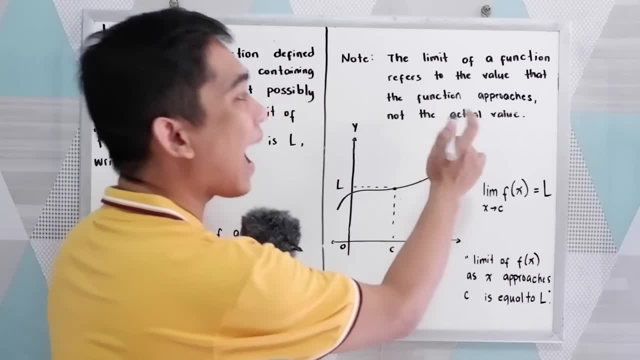 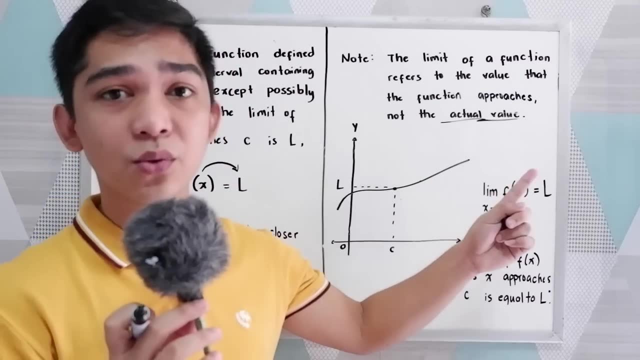 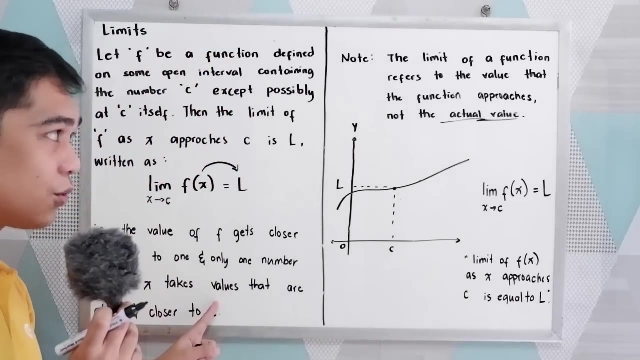 that the function approaches, Not the actual value. so take note of that, because if we're going, or if you're just going to get the actual value, that is the value of the function, but here in our limits, we're going to have the values as x. 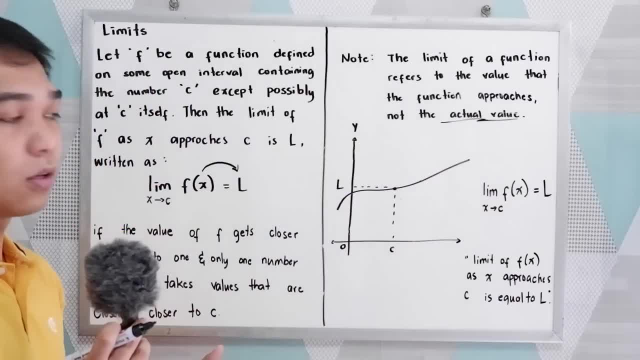 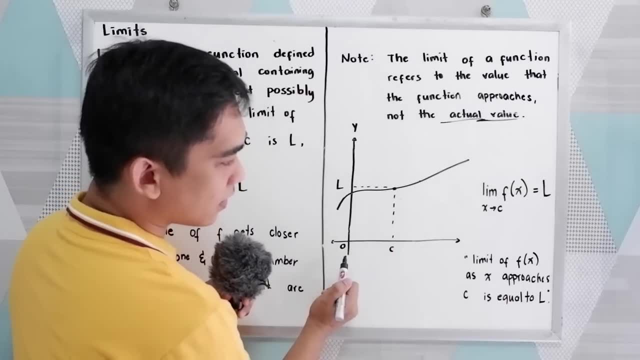 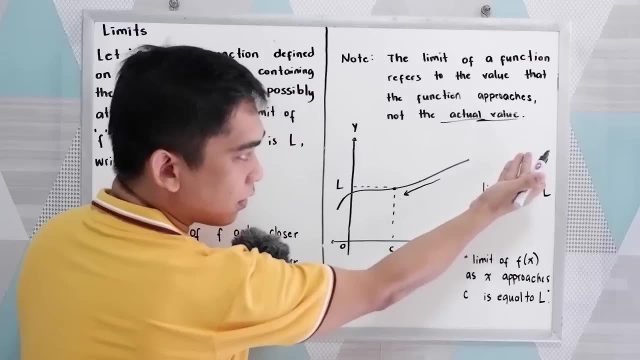 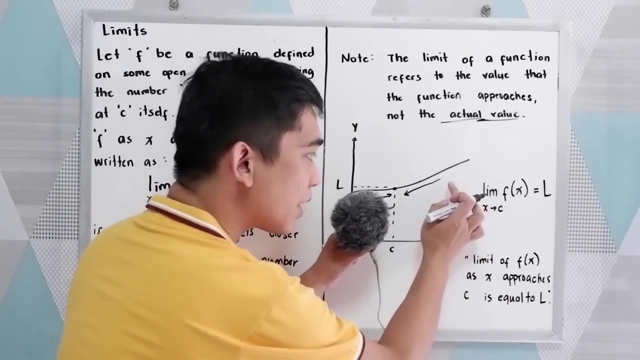 approaches to our constant. so to illustrate, let's have this graph. so we have here our constant, as we draw closer and closer to our constant. we have two areas here: from right going to left, then from left going to right, as we draw closer and closer to our. 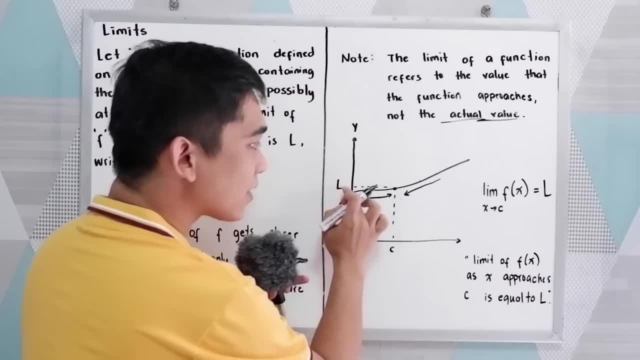 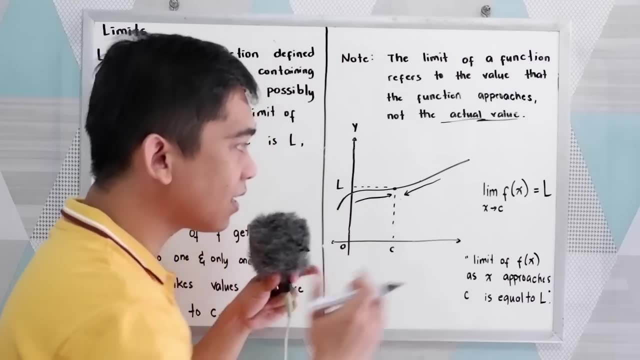 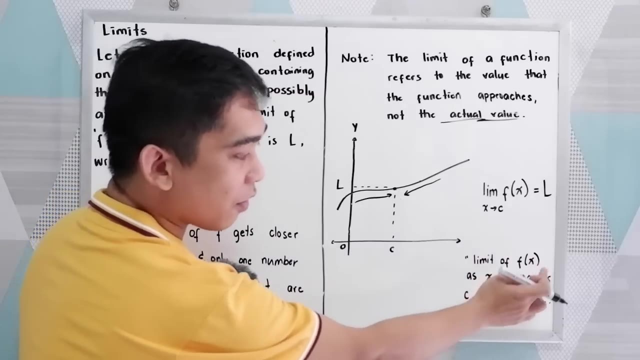 constant that will give us our l. okay. so the limit of f of x as x approaches c as you approach a c, that is equal to f of x to our L here. so that is read as the limit of f of X as X approaches C as X. 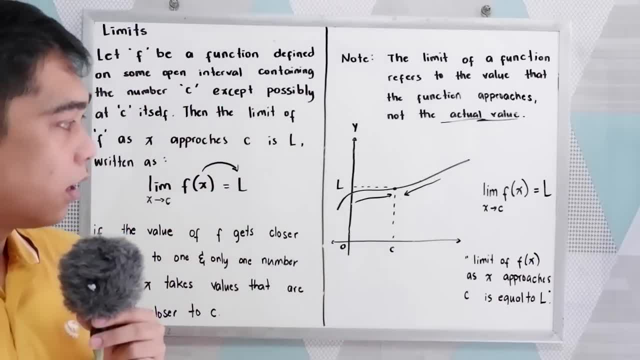 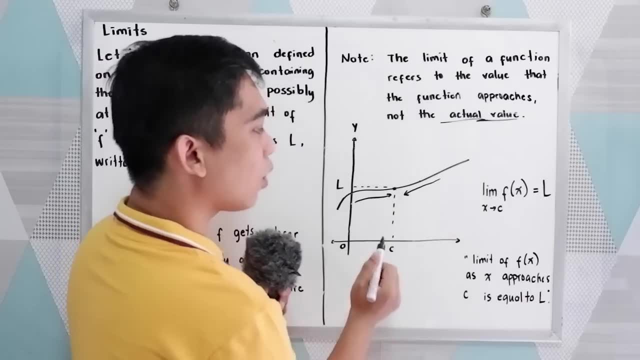 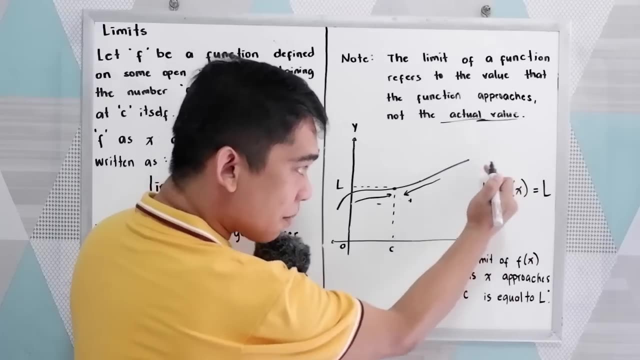 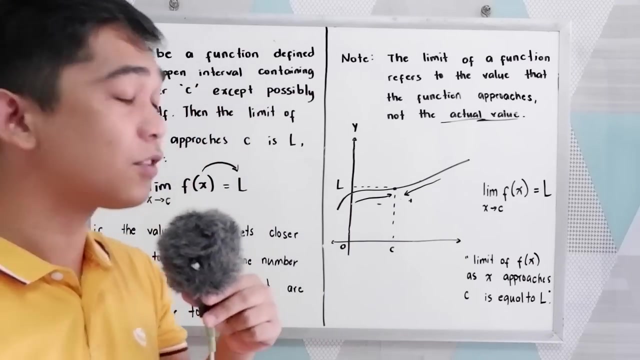 approaches, C is equal to L. so we are going to consider two areas: from the negative and going to, from the negative to our constant, then from the pasted numbers to our constant. okay, to illustrate and understand, let's have some examples. now, let's have our first example. 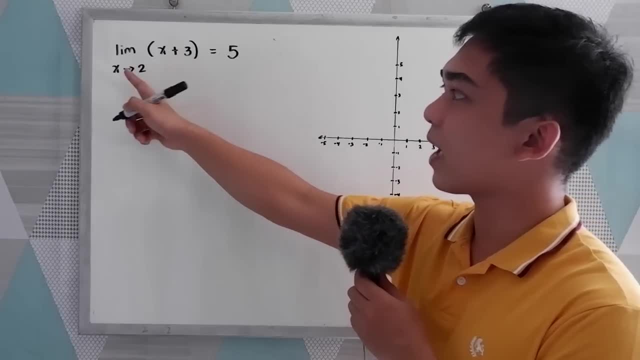 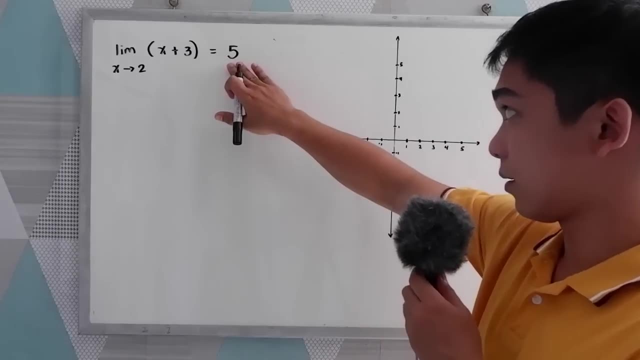 limit of X plus 3. as X approaches, 2 is equal to 5, so let us check our limit here if it is equal to 5. so again we have two areas that are equal to 5. so let's check our limit here if it is equal to 5. so again we have two areas that are equal to 5. so again we have two areas that are. 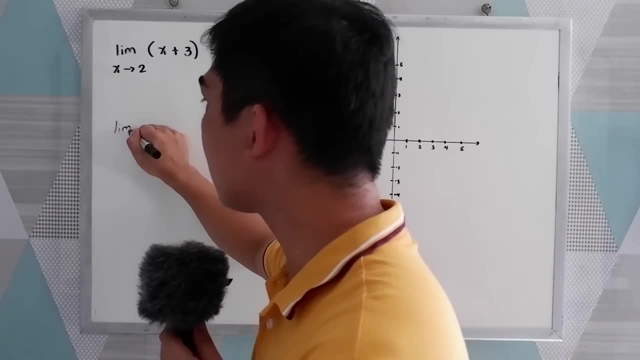 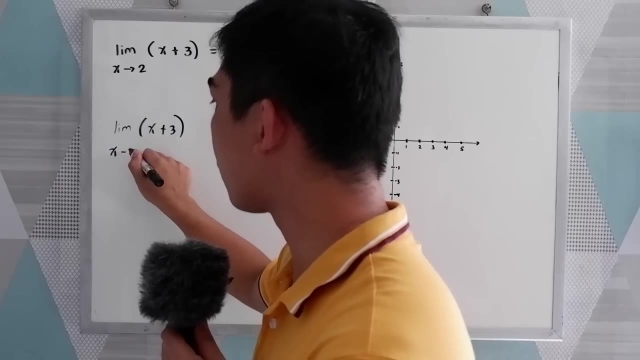 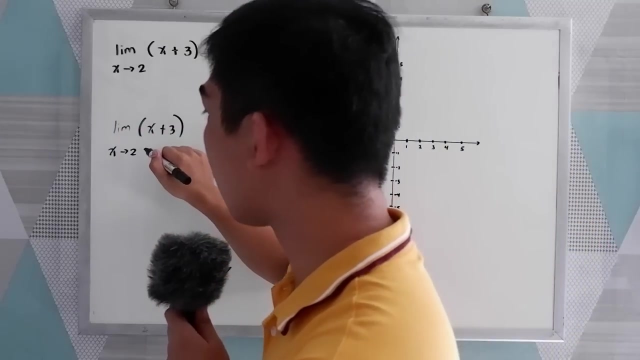 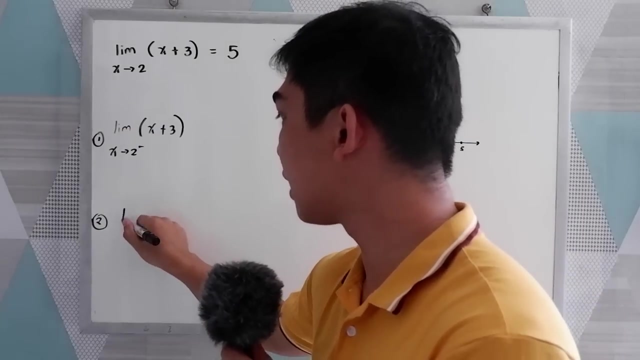 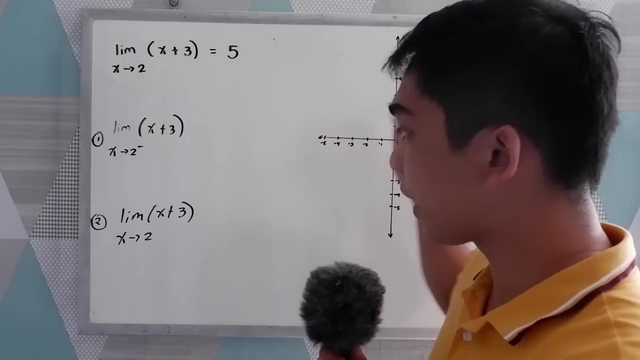 we need to consider. we have the limit of X plus 3 as X approaches 2. we have from the from the left side going to our constant, that is the negative, and the second one, the limit of X plus 3 as X approaches 2, from the right side going to our constant, which is 2, the positive in our 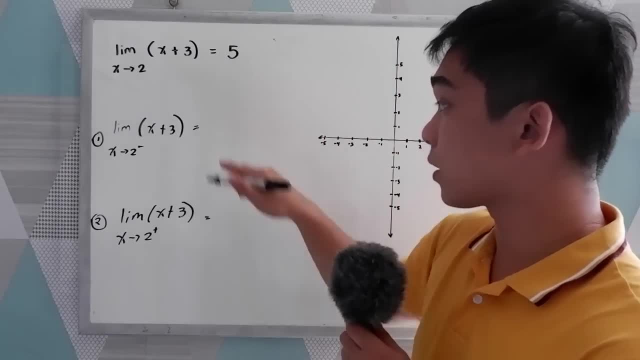 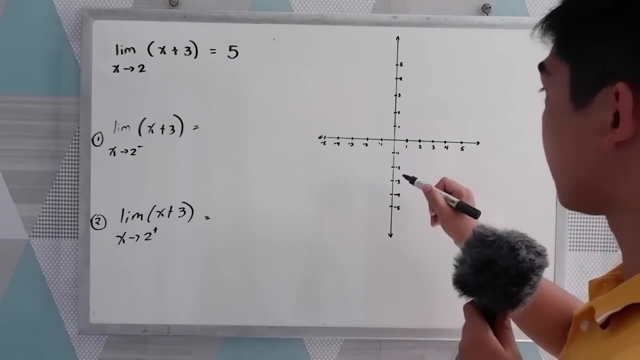 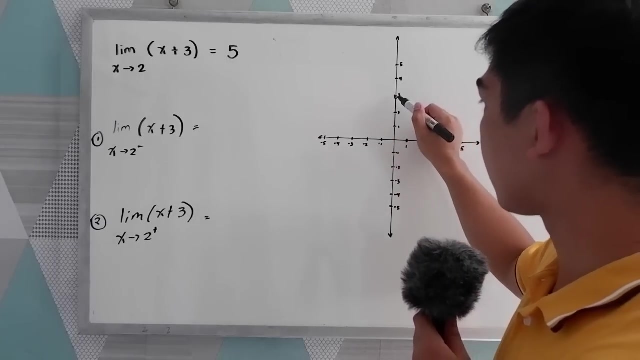 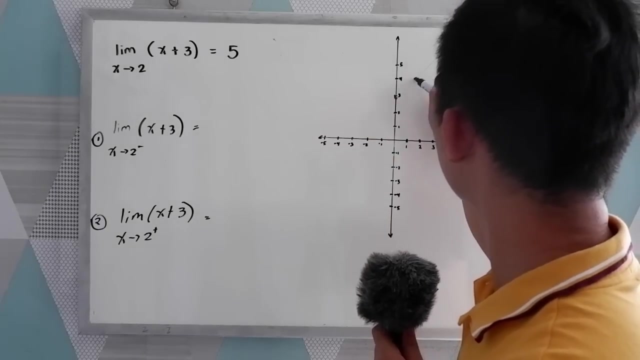 definition earlier, that must be equal to 5, so let us check. so first graph our function X plus 3, so our point here. then, if we're going to graph that, our slope is 1, so it could be like this one. okay, this would be hour. 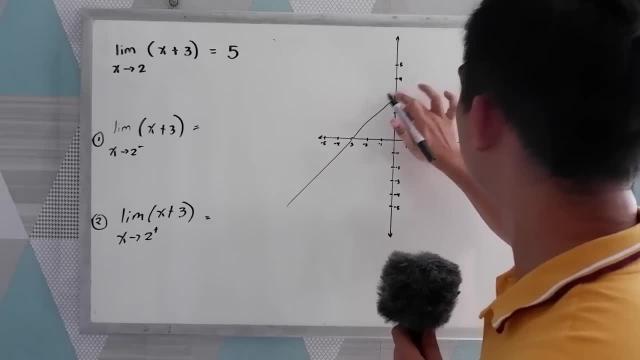 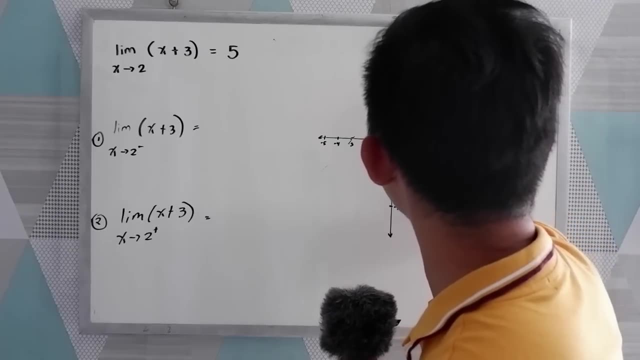 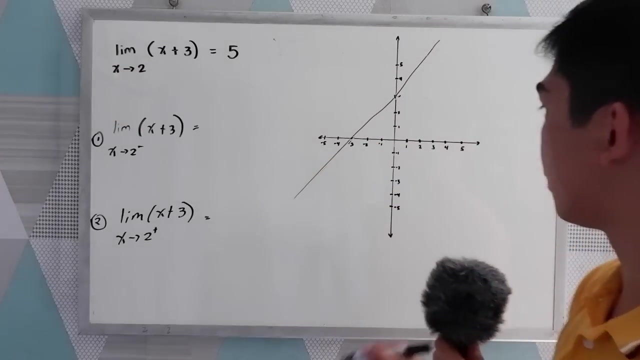 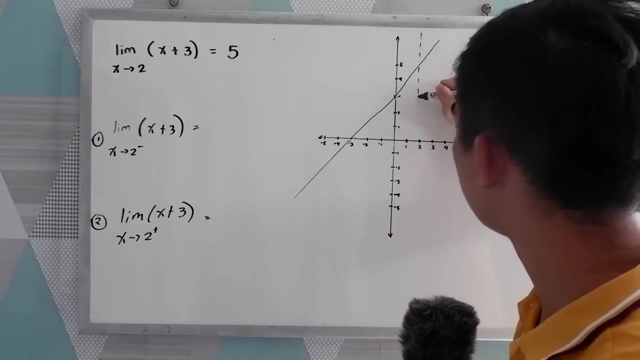 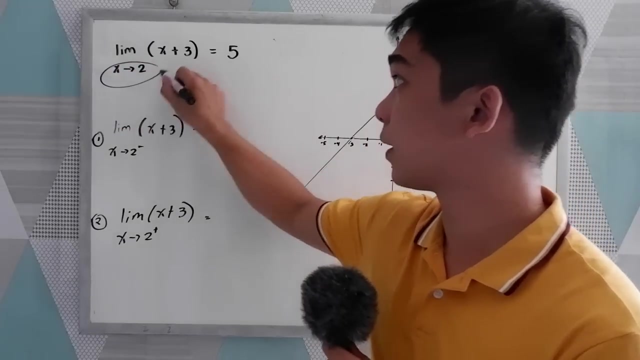 our line must be a straight line then as the ax approaches 2. so our bus, that is, 2 sockman wheel, seem to have vá wző MR 2021. our line- here we can use a broken line- our constant is 2 here. now check our. 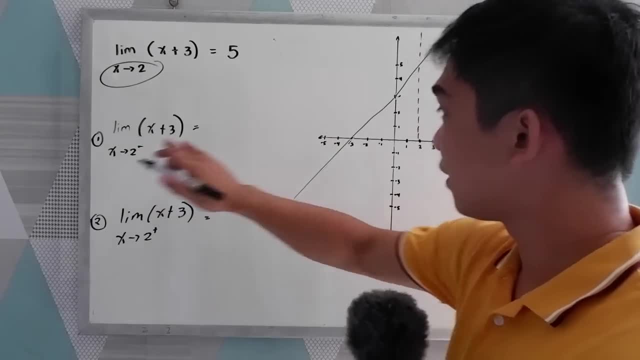 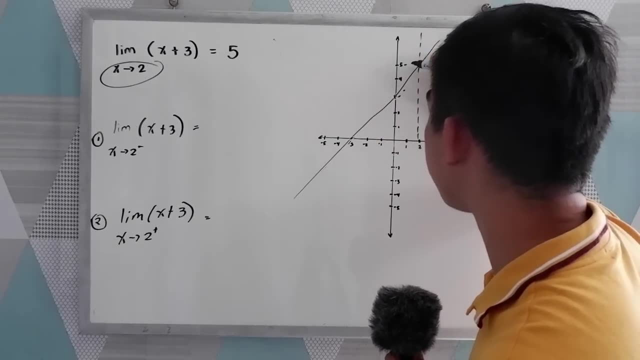 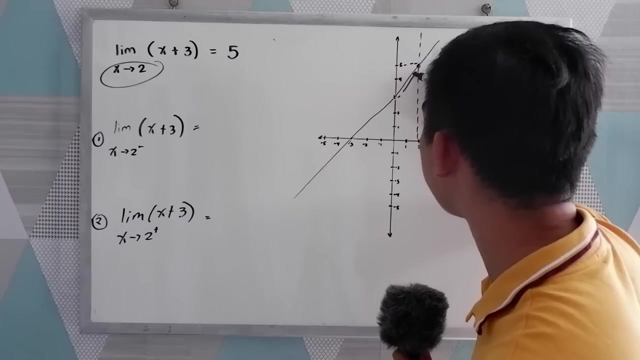 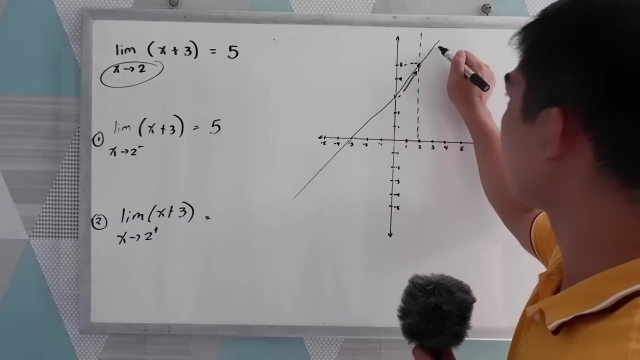 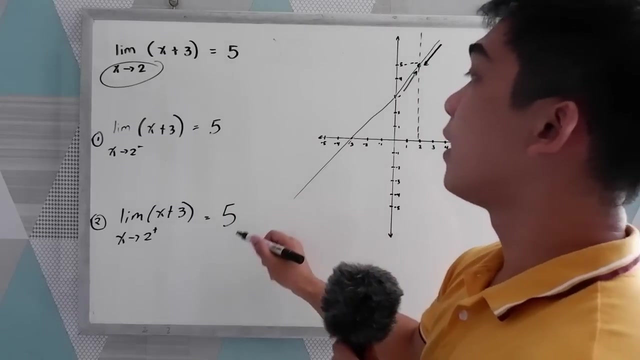 graph. let's start with the from the negative or from the left side, so going to our L. so our end here is 5. so let us verify our point is here. so okay, correct, that will give us 5. and the other one from the past team go into our constant. that will also give us 5 again, the number L or our L. 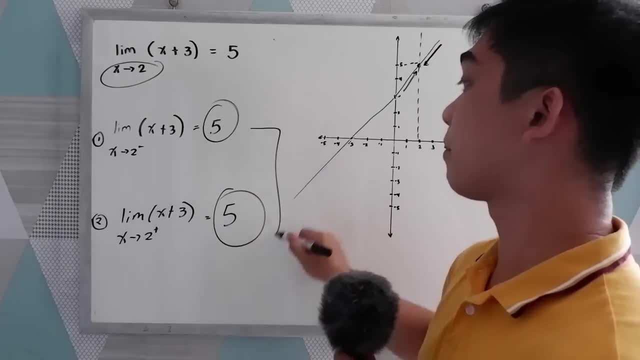 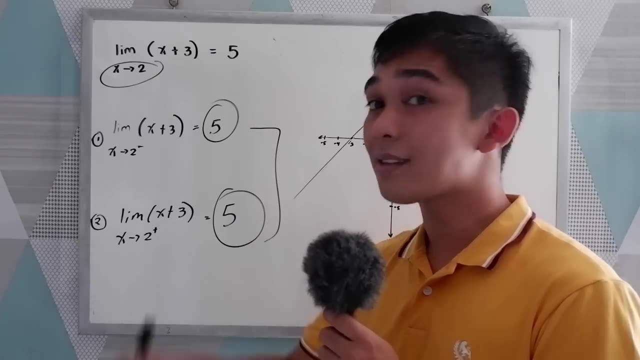 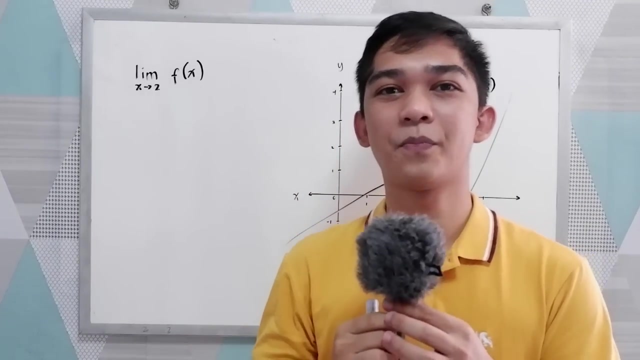 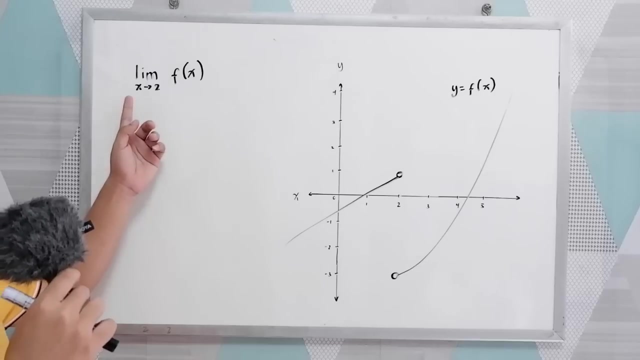 must be one number or they must be the same. If they are not the same, that will give us does not exist. So let's have example for that. Now let's have our second example. Let us use this graph to find the limit of f of x as x approaches 2.. 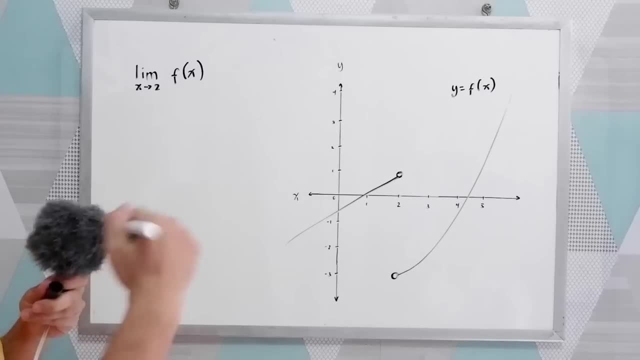 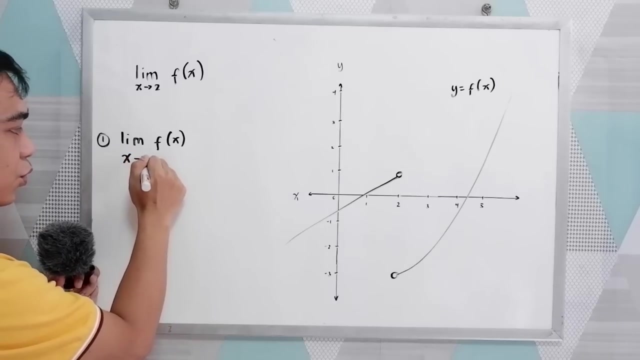 So we need to consider our two areas. First one is the limit of f of x of our function as x approaches 2 from here to the left. that is the negative. And the second one, the limit of f of x as x approaches 2 from here to the left. that is the negative. 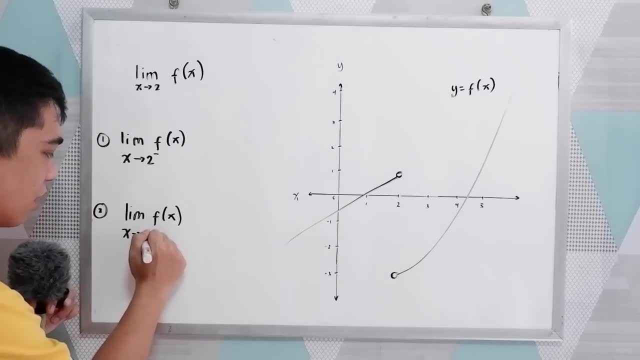 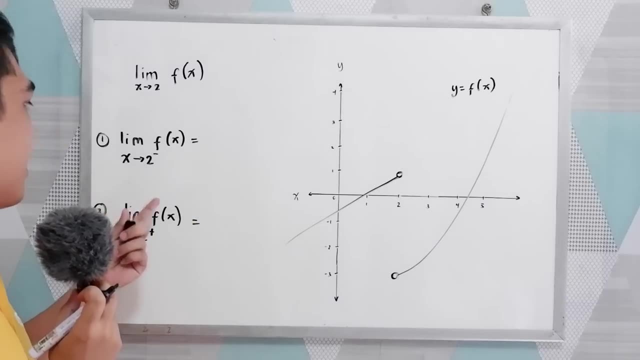 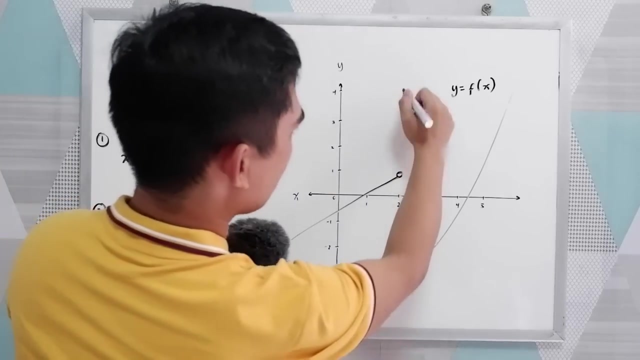 The second one, the right side, the positive. Now let's find first our first one: the limit of f of x as x approaches 2.. So our constant is 2.. This is our constant, So our constant. we drew a broken line. 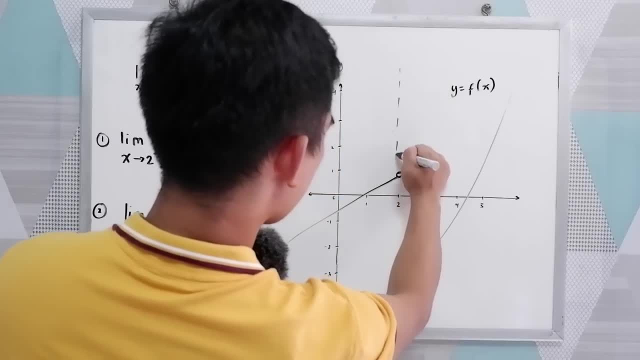 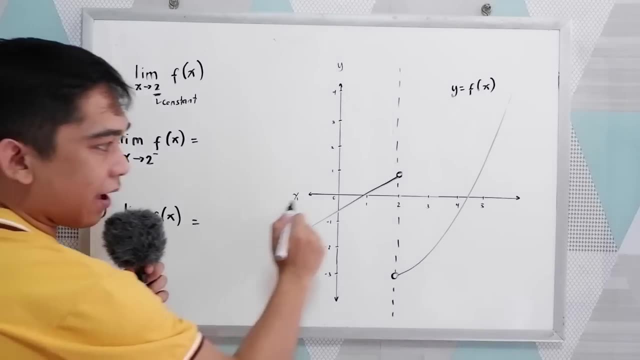 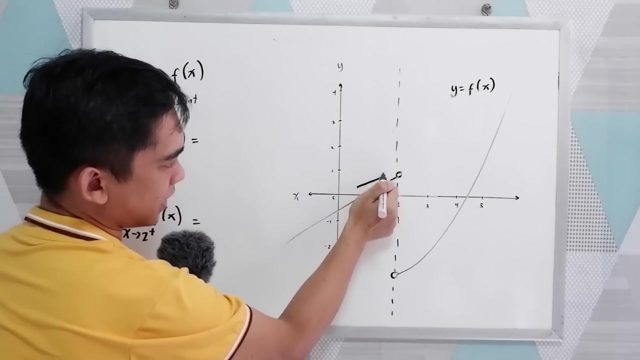 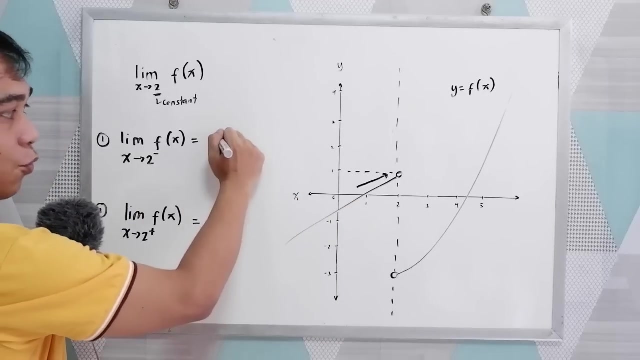 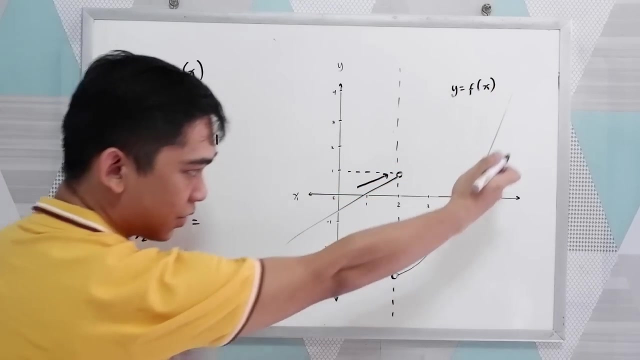 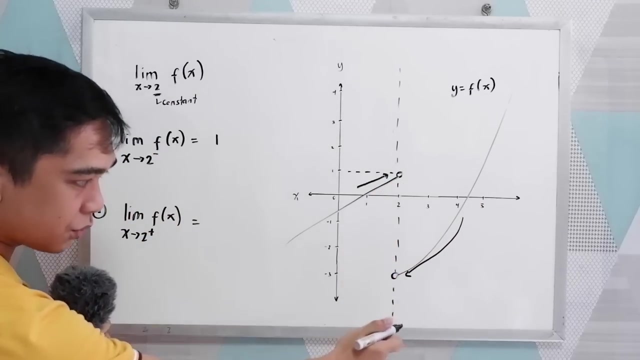 So our 2.. Okay Now, from the left, going to our constant, as we approaches to our constant, this will be our L, That will give us positive 1.. And From the right, going to our constant, as we approaches to positive 2, this will be: 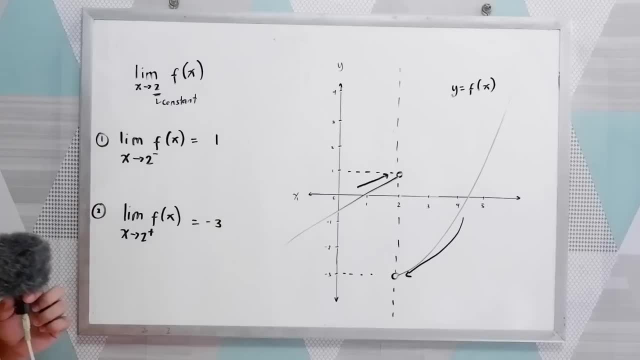 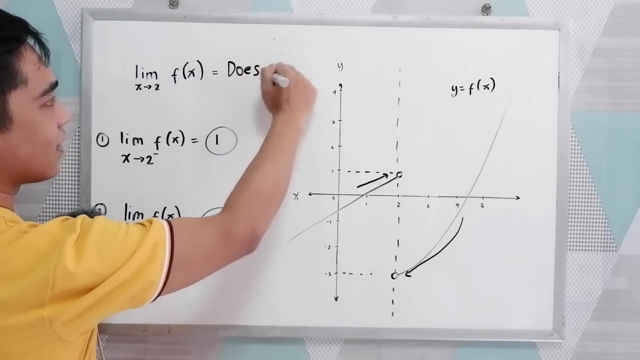 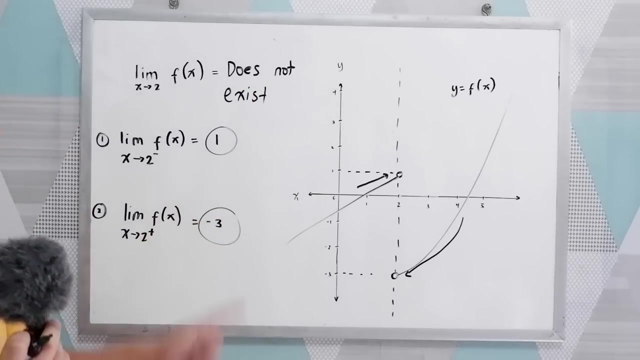 our L that is negative. 3.. Notice that our L or our limit are different. So therefore, the limit of f of x, As x approaches 2, does not exist because, according to our definition, this 2 must be. 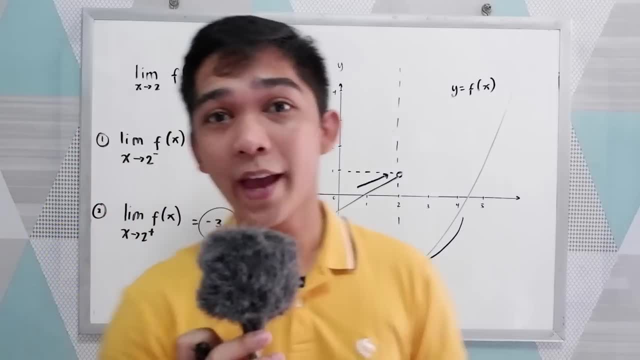 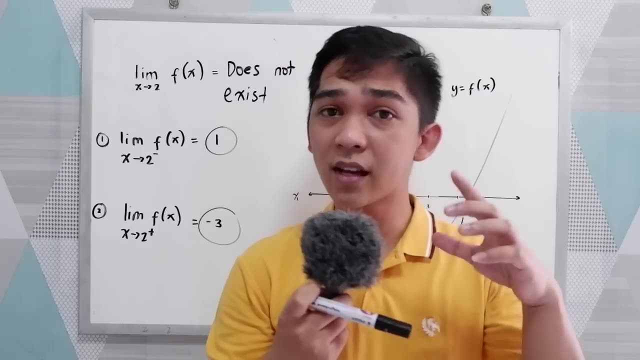 the same. So that is the application and the definition. Thank you for watching Senior Pablo TV. For our next lesson, we're going to discuss the theorems on limits.